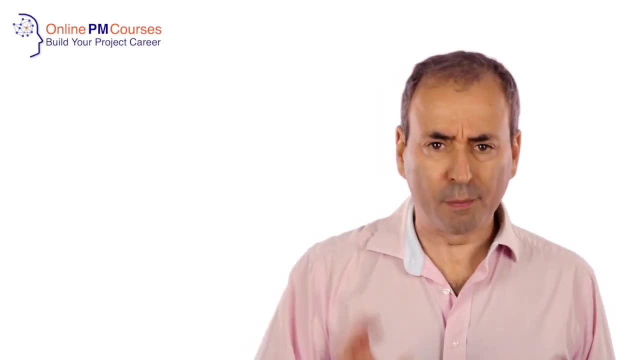 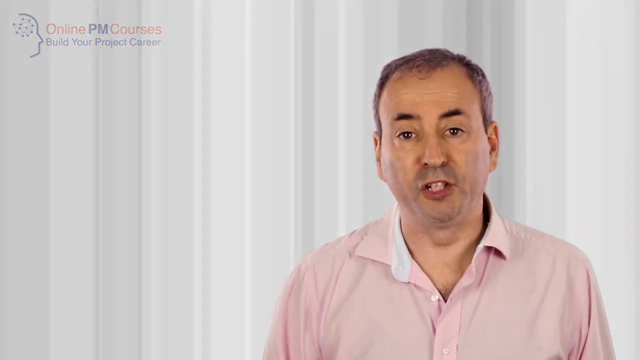 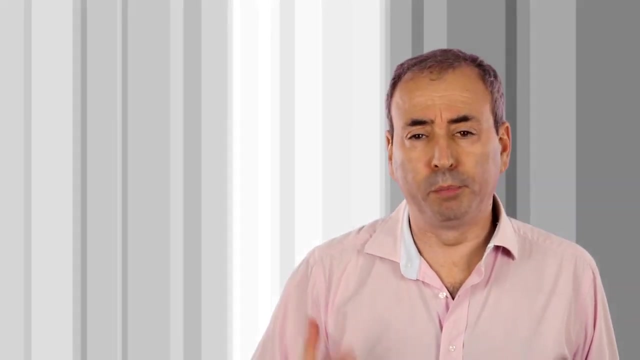 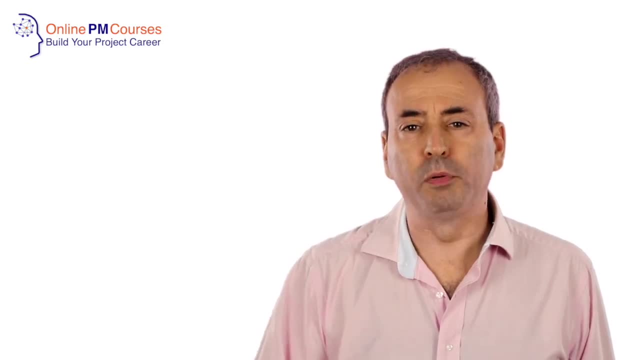 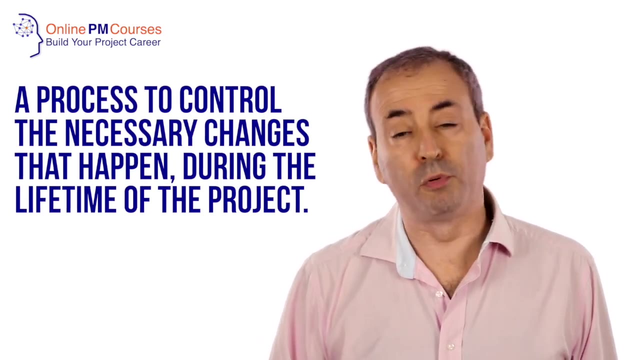 And then we stuck in the middle of it, And then we stuck to it rigorously. Change control therefore provides us with a process to control the necessary changes that happen during the lifetime of a project. Now, of course, what happens on a project typically? 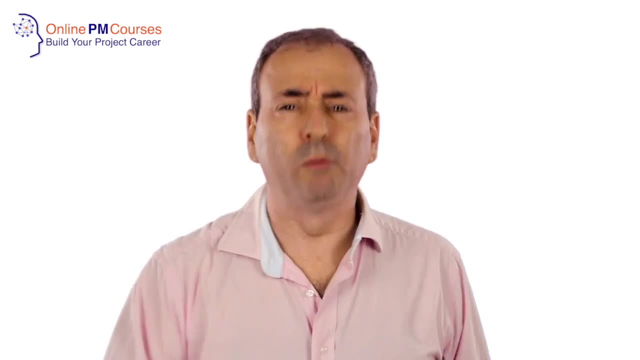 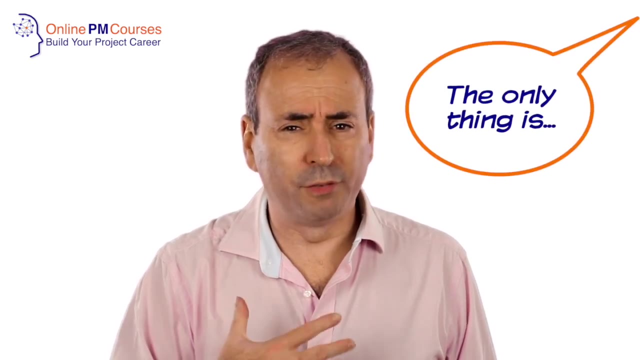 is that things are going well. And you know they're going well because that's when someone comes up to you and says, hey, Mike, everything's going great. The only thing is we've- I've, you know- changed our minds. Now, as a project manager, 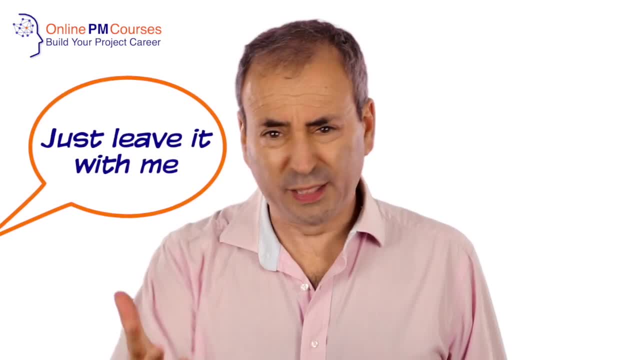 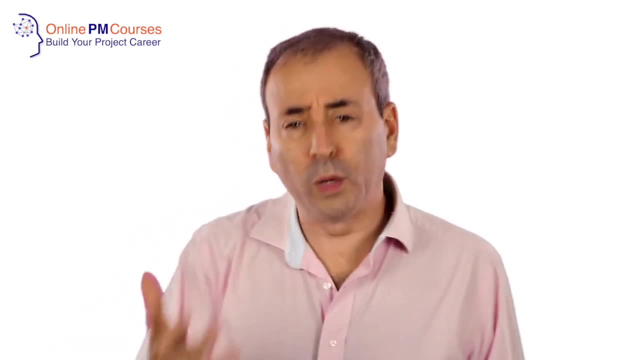 your first instinct is almost certainly to say: oh, it's fine, Just just leave it with me, I'll sort it out, Just do it. But of course the problem with that is: where's the budget coming from for the extra work? Where's the time in the schedule going to come from? Where are you going? 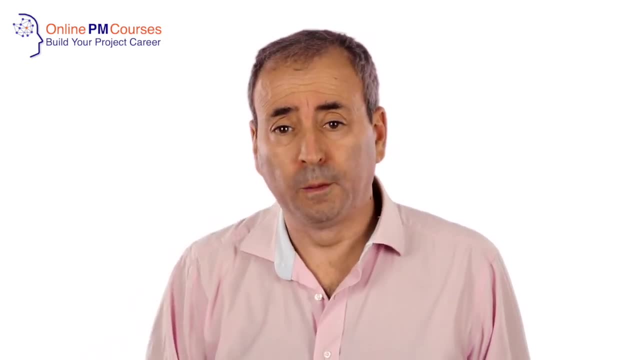 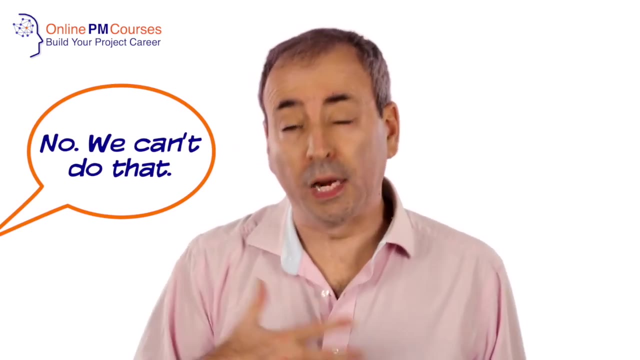 to get the resources from? And what about all the additional risk? Perhaps it's safer to say: well, no, we can't do that. We've signed off our definition, We've signed off our plan, our specifications, We can't change anything. But of course, as we've seen, sometimes you need to. 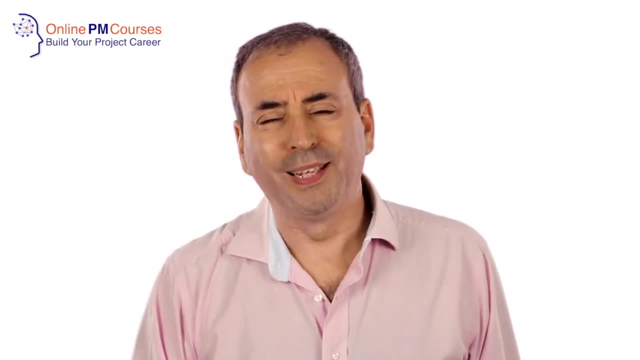 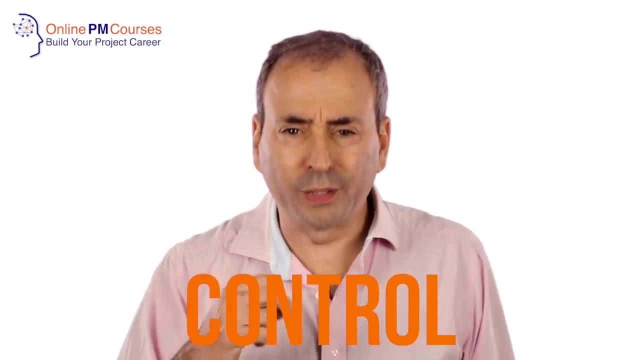 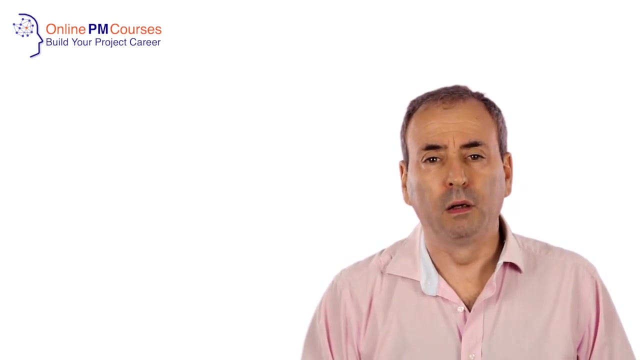 So what do we need? We need the one thing that project managers crave above all else. We need control And a change control process is what gives us that control, And it's a very simple process And it starts with that question: Change my mind, I want to. 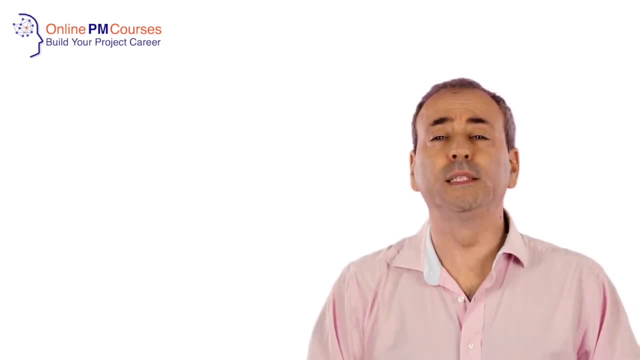 do something different, And your answer to that isn't yes and it isn't no, It's thank you. And then you ask the person who's come up with the idea for change to document the two things They are best suited, best able to document. firstly, what precisely is the change that they're asking? 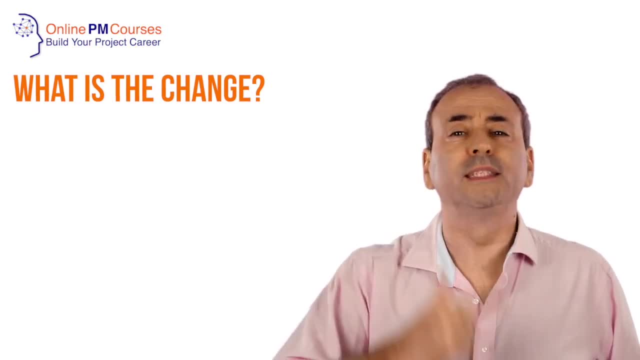 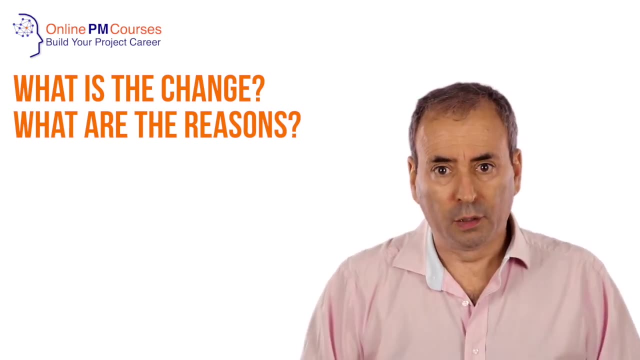 for Because you can't do anything until you know what it is they want. And secondly, what are the reasons why they believe this change is right? Is there a compelling, necessary reason to make the change, Or is there a compelling advantage and benefit in making the change Now, once they've? 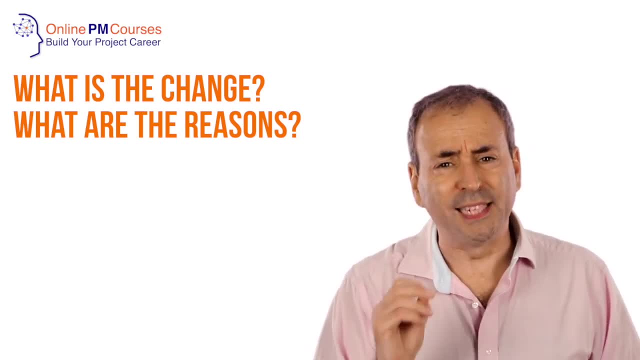 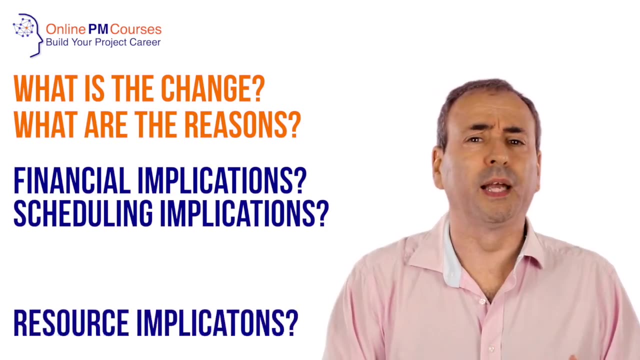 done that, you can take that clear articulation of what the change is And you can then work out what are the financial implications. What are the financial implications? What are the financial implications? What are the schedule implications? What are the resource implications? What are the 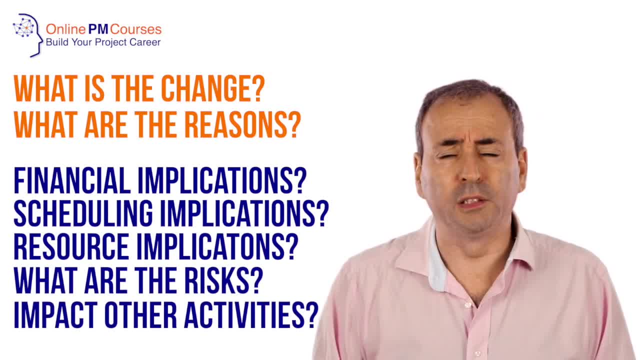 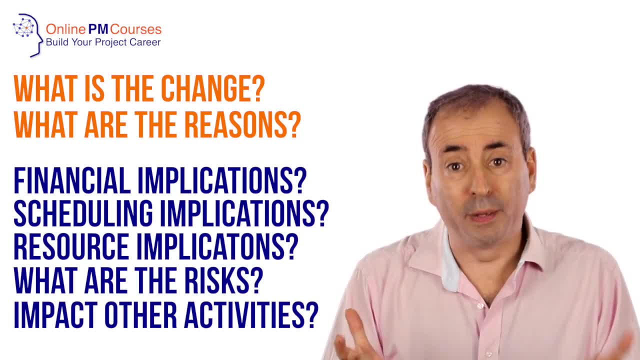 risks that arise from it And how does this impact other things that you know are going on outside of your project. And when you've got all the reasons why you should change and all the implications of change in terms of budget and schedule, risk and impact, then you can take them to your decision. 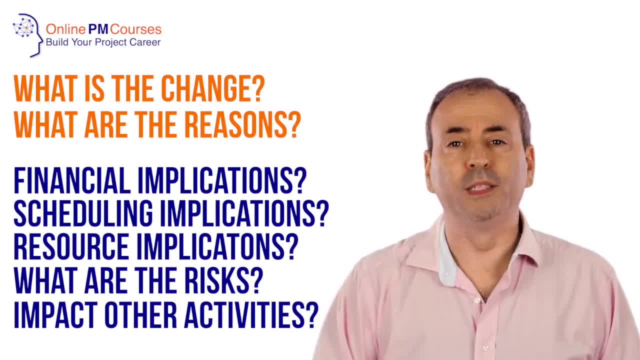 makers And they can make an informed decision, And that's either going to be to accept the change or to reject the change. And that's either going to be to accept the change or to reject the change. And that's either going to be to accept the change or to reject the change. And the only reason why. 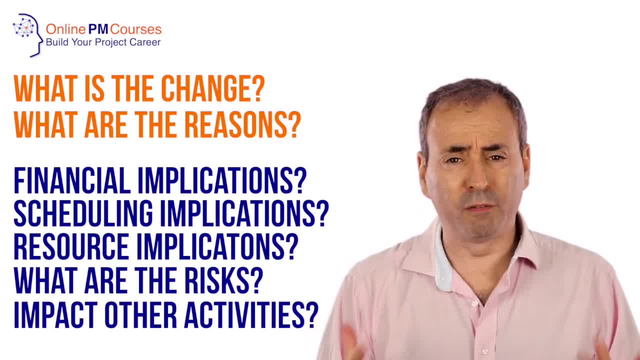 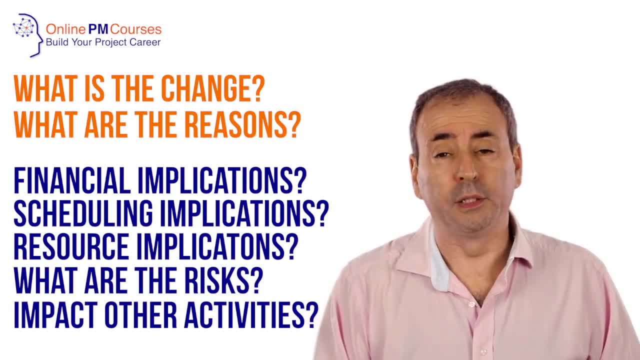 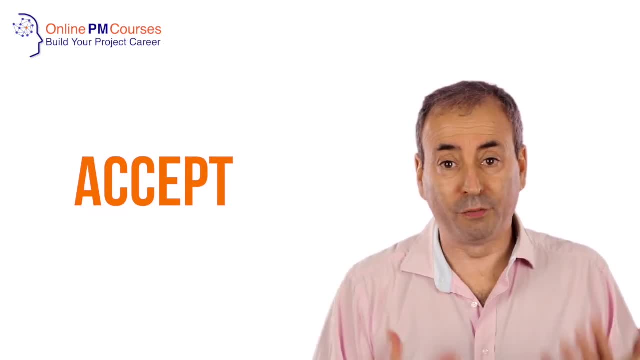 they might defer a decision is because they believe that you haven't provided them with all the information they need to make a decision, in which case you have failed to a degree in your job. So if they decide to accept it, your stakeholder is happy because they've got what. 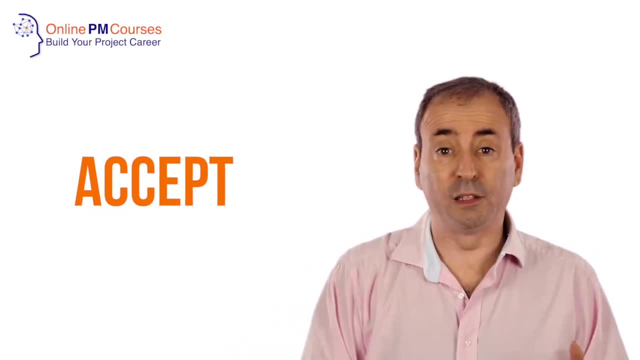 they want And you're happy because you've got the extra budget, you've got the extra time in the schedule, you've got acceptance of the risk, you've got access to the resources you need, you've done the planning. It's just a job. 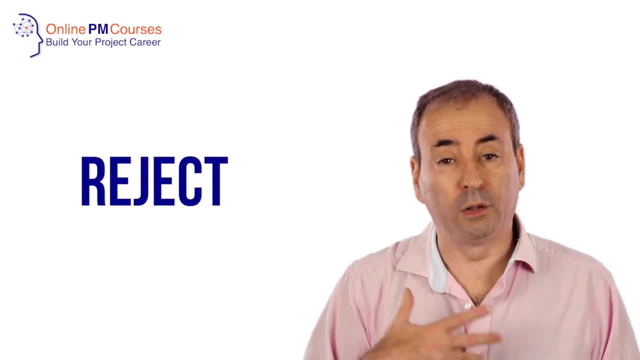 If, on the other hand, the decision is no, it's too risky, it's not enough benefit, or whatever, then that's it. I'm afraid The stakeholder who asks for the change is going to be I am sure. 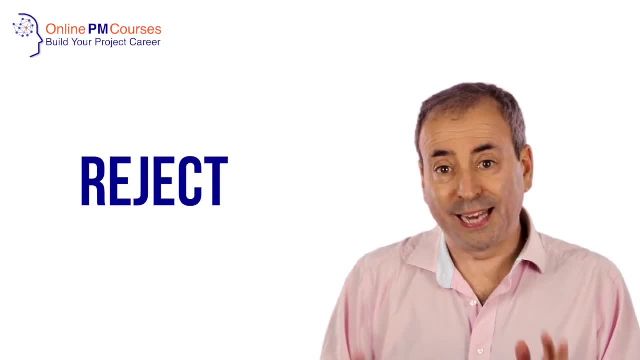 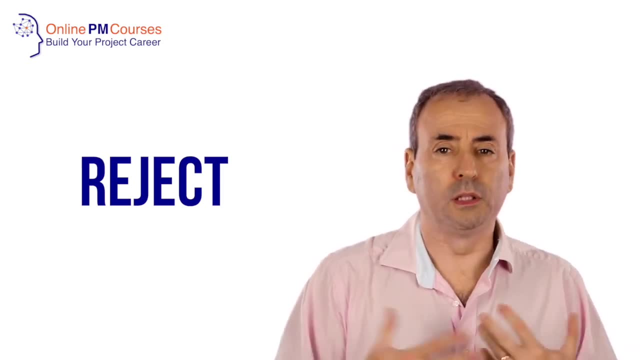 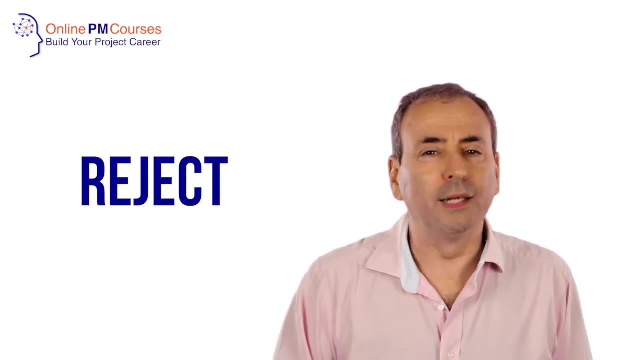 disappointed And many change control processes actually have a stage within them where the stakeholder can advocate in person to a board or a design authority group that makes the decision. They may be disappointed, but at least they know that this isn't you, the project manager being. 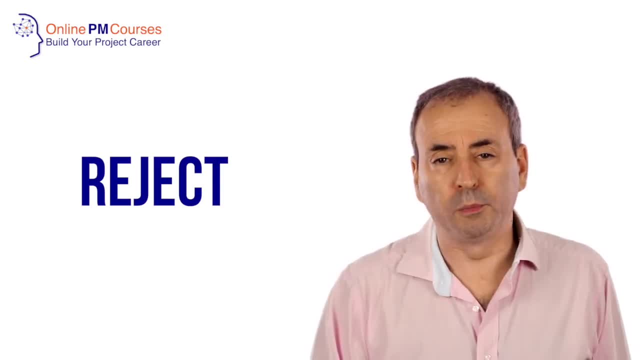 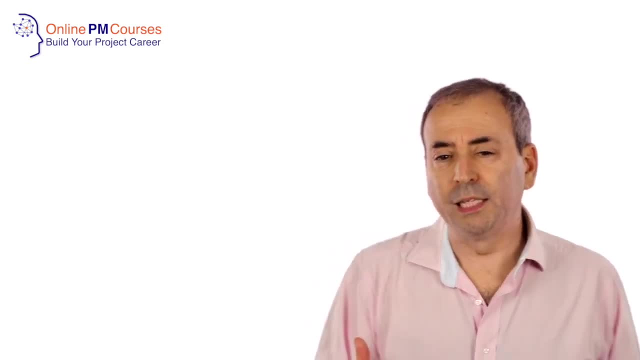 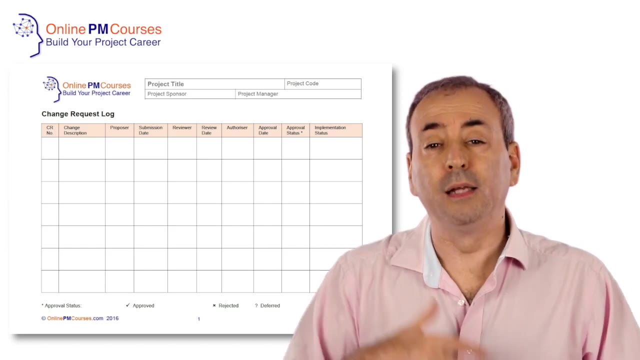 capricious. There's been a robust process and it's auditable, But that's it. No change. Now, when there is a change to be made, or whether there isn't a change to be made, every request goes into a change log which details the request that's made, the timings.